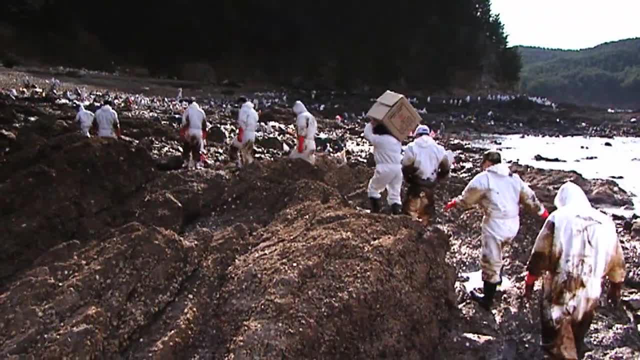 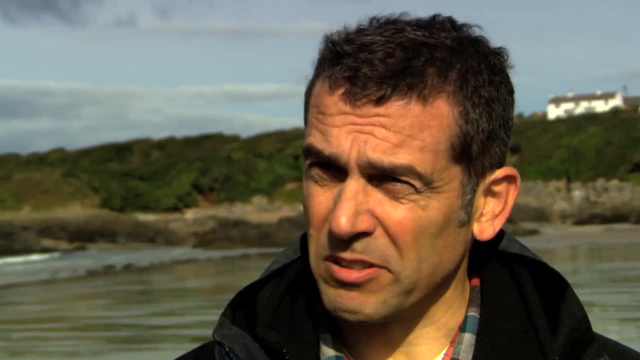 environmental catastrophe. What issues should be considered, from the type of oil spilled- Forewarned is forearmed- I mean the millions, I mean in military terms, it's know your enemy- to the techniques available for clean-up. 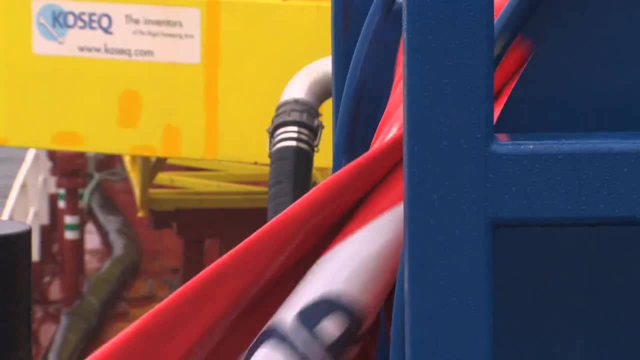 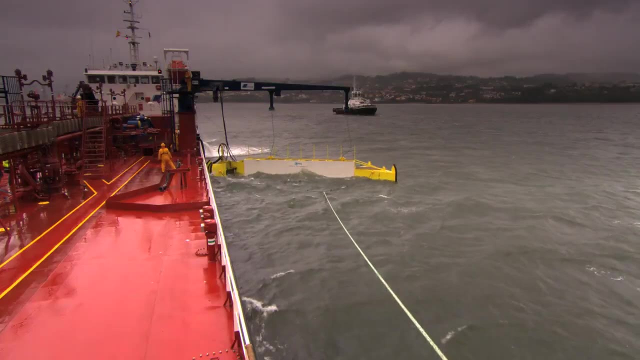 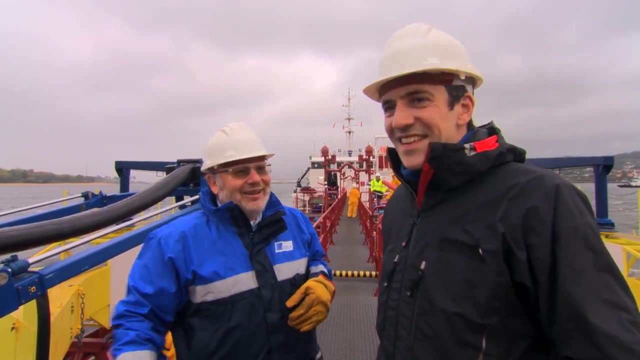 This vessel has state-of-the-art equipment In a real spill, 50% of the equipment you don't need. But if you could tell me on the next spill which equipment I need, you'd get a contract with me, I see. 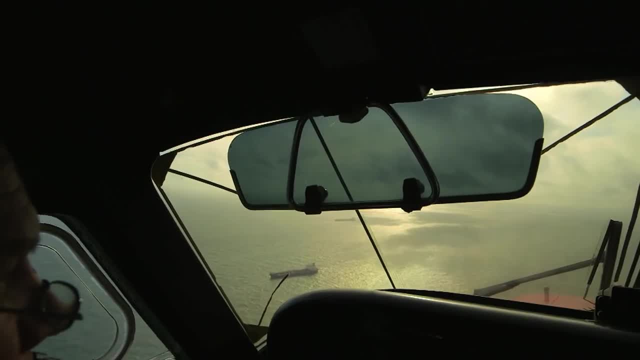 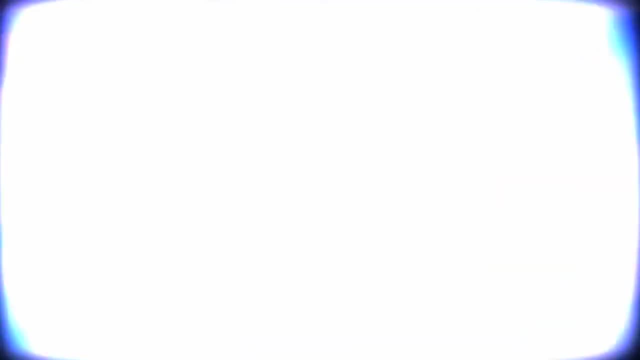 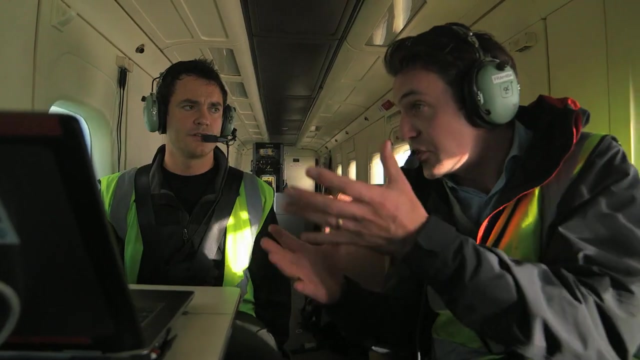 I'll be finding out how to plan for an oil spill, how to prepare for an oil spill- You can save precious moments right at the outset of a spill, when the damage is potentially the greatest- and how to respond when one strikes Overall, how important is it to get up here? 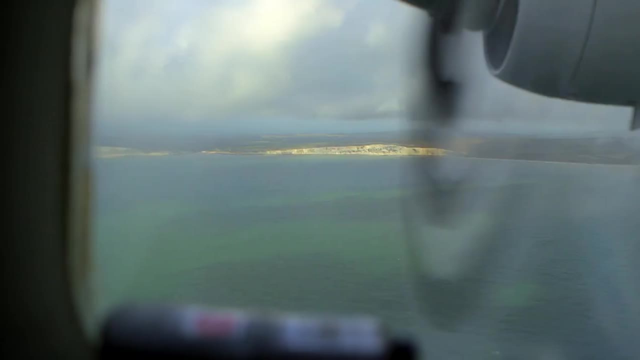 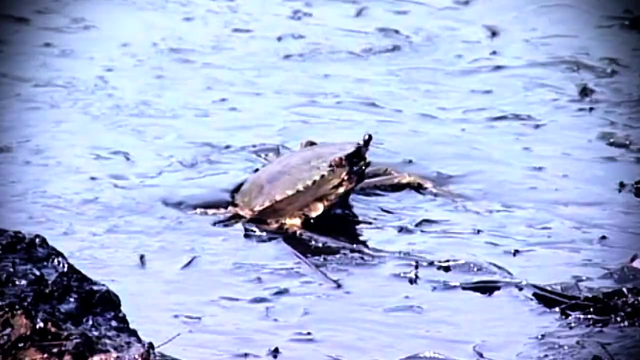 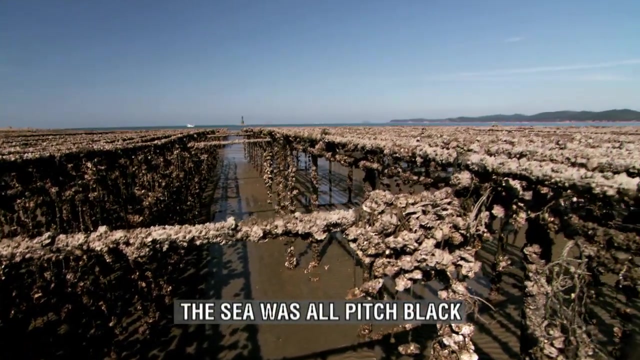 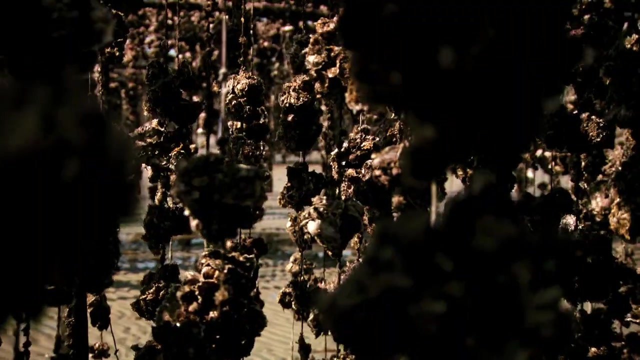 and actually get a view of the oil from above. It's the only way really to get the very good quality information about the resources at risk. I'll look at the environmental and economic impact of spills around the world and the systems in place for compensation. 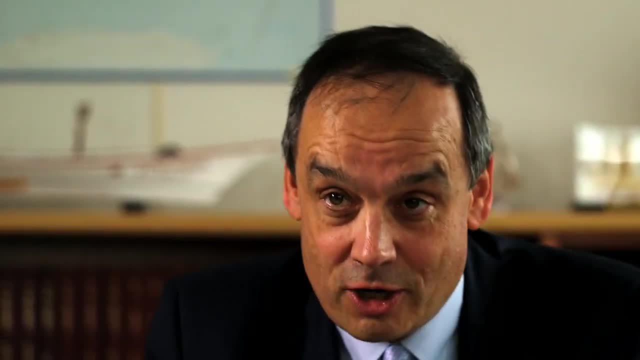 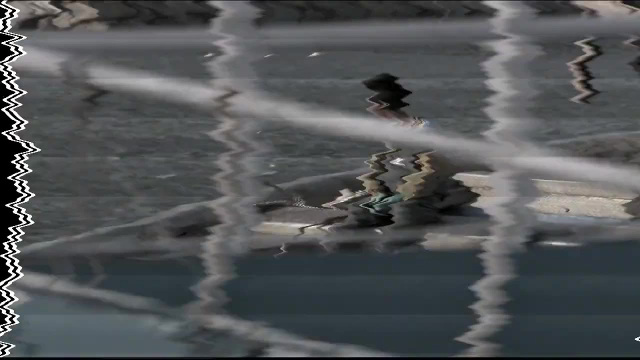 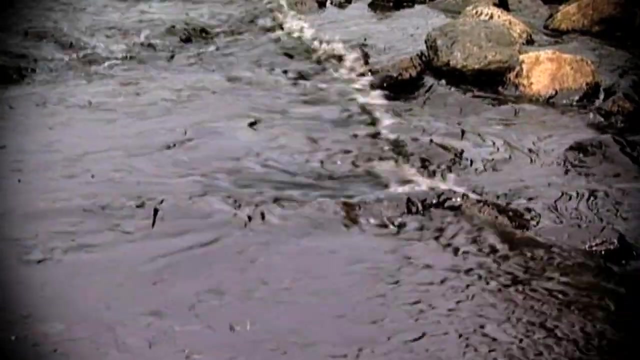 We have a legal framework, we have the money available, we have how to sell it and we've advanced quite a lot in 35 years. And I'll be asking: whether it's at sea or on shore, how do we deliver a well-planned and executed response? 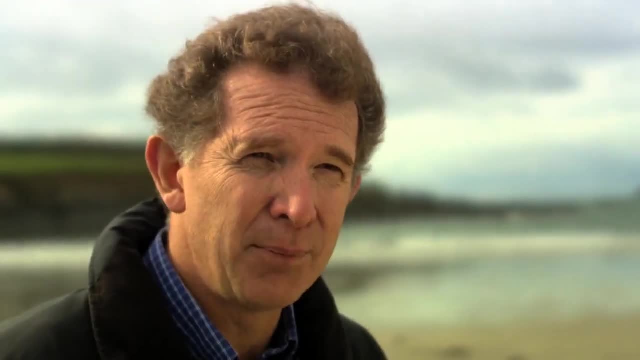 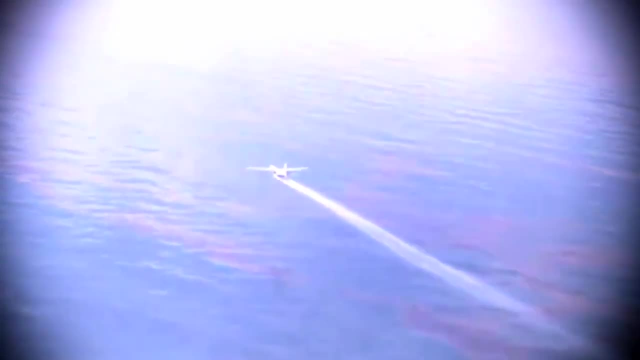 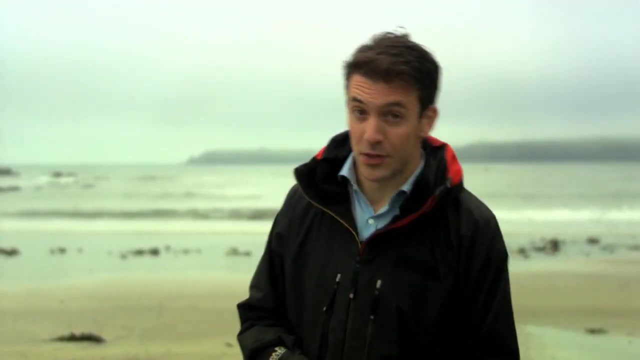 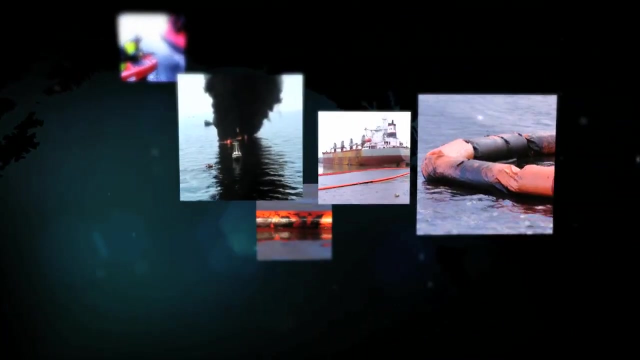 to mitigate damage. It's really important to know the advantages and the drawbacks from different techniques so you can minimise the impact. Accidents will happen. What's important is to be ready for them when they do. When you do, you know what it's like to have a window on yourself. 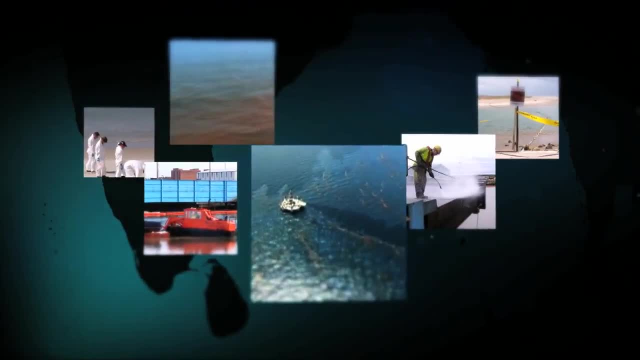 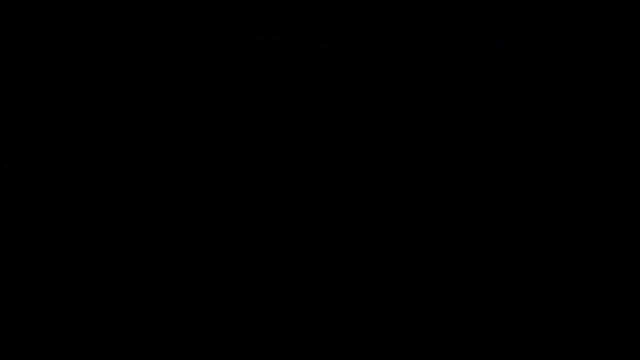 It's great to be able to see that you're not alone. TensorFlow is a great tool for us. How do you support yourself? cosmosorg sourcegov, Powered by TIPS. wwwtigovau, wwwtigovau, wwwtigovau. wwwficom, wwwficom, wwwficom, wwwficom.